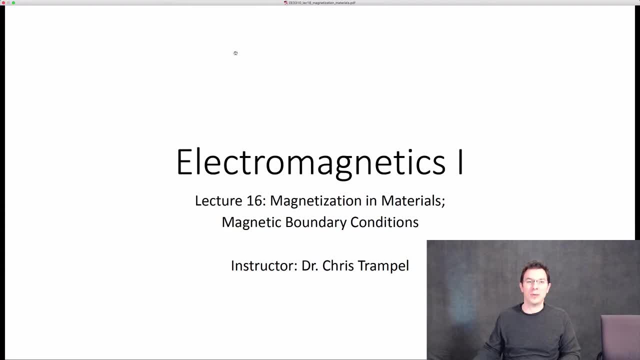 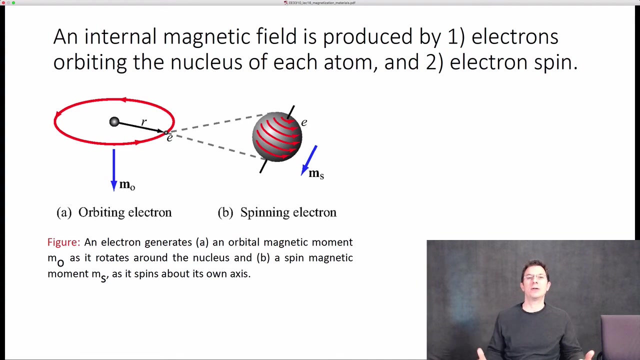 Hello and welcome to Electromagnetics 1.. Dr Trample here. This is lecture number 16.. Today we're going to be talking about magnetization of materials and magnetic boundary conditions, So two pretty big topics. Well, how is it that some materials in nature respond to the magnetic field and others don't? Which is to say, what is the microscopic origin of magnetic response? 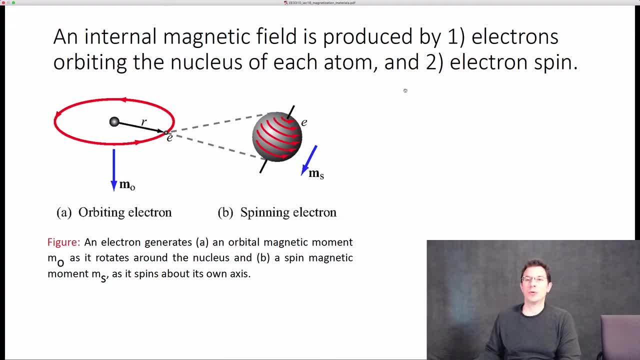 Well, an internal magnetic field is produced in two ways. The first is by electrons orbiting the nucleus of each atom. That's shown here in this figure. You can see that you've got an electron orbiting a positively charged nucleus which creates a magnetic field. 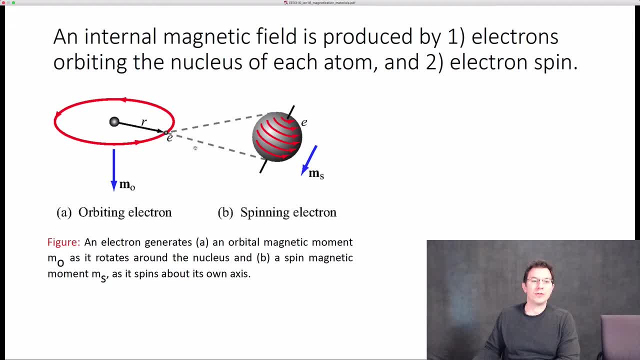 And then also, if you sort of zoom in here, on the electron itself. the electron itself is processing or spinning, And that spin itself actually also creates a magnetic field. So the magnetic field in a material occurs in two ways: Because of the orbiting of the electron around the nucleus and because the electron itself is spinning. 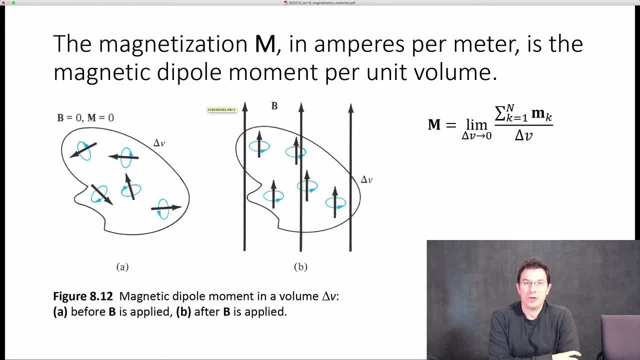 The magnetization vector capital M, which has units amperes per meter, Is the magnetic dipole moment per unit volume. On the left hand side, here in this left figure, you can see a material, and each of these little loops with an arrow is like an atom or a molecule or something like that. 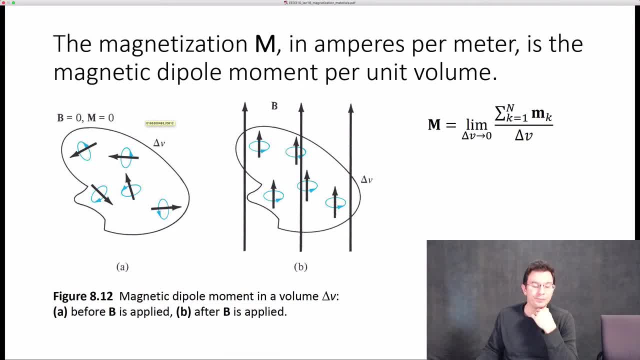 And you can see that, in general, in most materials, the magnetic dipole moment, as indicated by those arrows, is oriented in a random fashion. However, if you were to apply an external magnetic field to this material, each of these, the external magnetic field, actually causes each of these loops to feel a torque, and we'll talk about that in a moment. 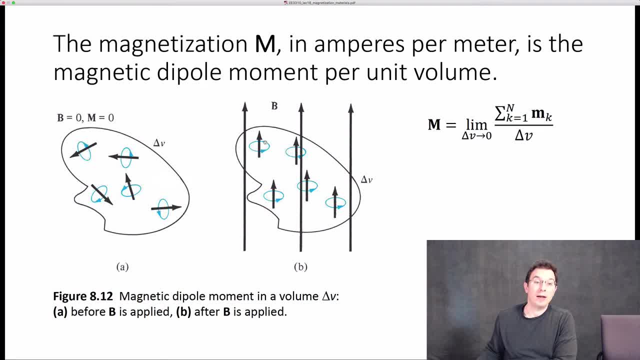 And they all line up. they all tend to line up with the external magnetic field. The important thing here is that we can characterize how well or how strongly this happens in a material using this magnetization vector, capital M. Mathematically we'd say that M is the sum over all of these little magnetic dipoles here, however many you have. 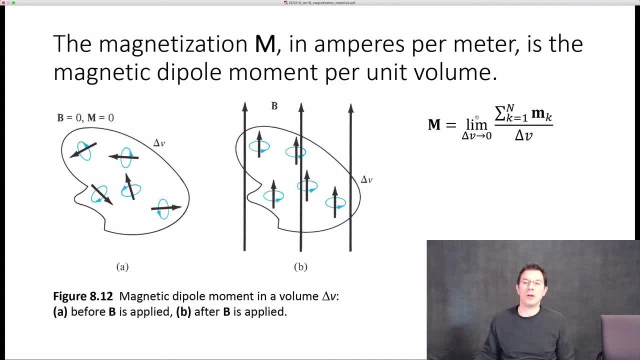 You add those all up vectorially in a small volume and you divide by the size of the volume and then you take the limit as the volume goes to zero And that tells you how much you'll be able to magnetize the material. essentially, 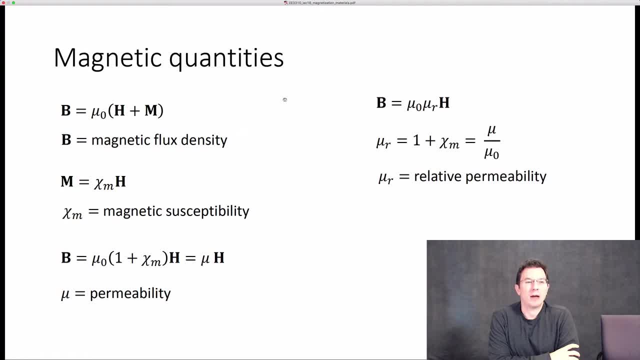 Okay. well, we've got a whole bunch of important magnetic quantities here that we need to discuss. The first one is the magnetic flux density capital B, And mathematically we say that the magnetic flux density B here is equal to the permeability of free space. mu naught. 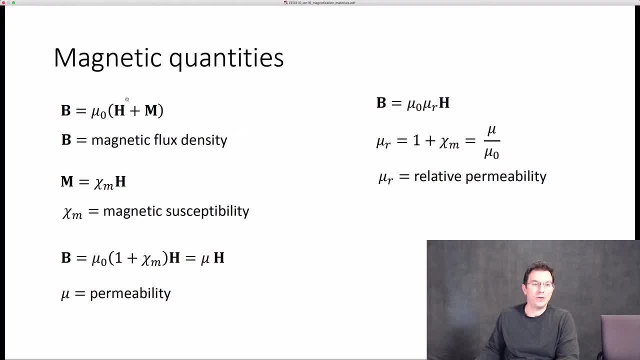 times the sum of the magnetic field and that magnetization vector capital M. We can usually relate the magnetization vector capital M to the magnetic flux density capital B, And the constant of proportionality here chi sub M is the magnetic susceptibility. So we can come back in here to this expression. substitute chi M H in for capital M. 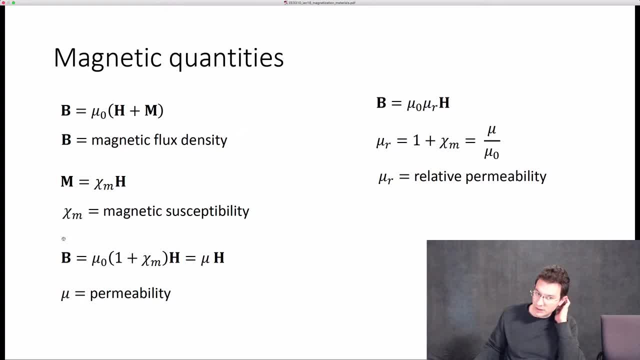 and we get this expression for the magnetic flux density. It's equal to mu naught times one, plus the susceptibility times, the magnetic field, And we can gather all of these terms into single coefficients. So we have a coefficient that we call mu, which is the permeability. 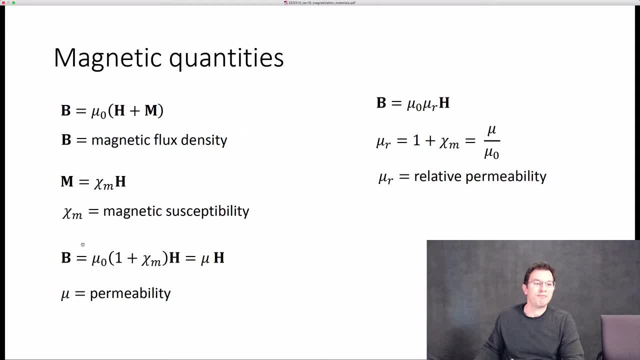 So mu naught is the permeability of free space, Mu is the permeability of a material. If chi sub M is non-zero, you have a magnetic material. In other words, the material is going to respond to the magnetic field. A couple more definitions here. 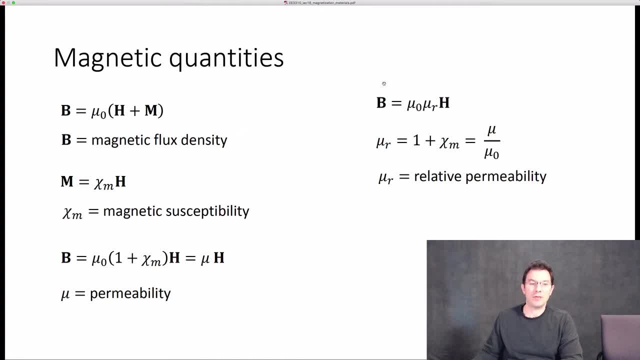 We can further break this out and say: the magnetic flux density is related linearly to the magnetic field by the permeability of free space times, mu sub R, which is called the relative permeability. And the relative permeability is given by one plus the susceptibility. 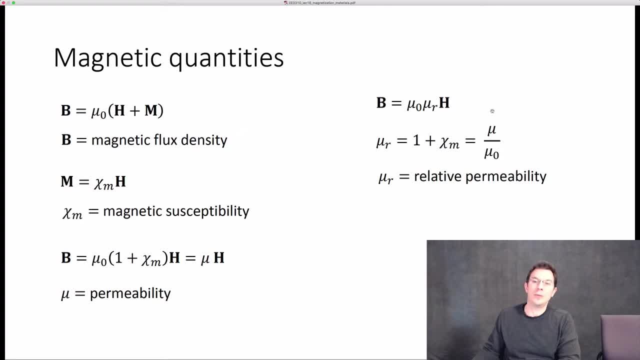 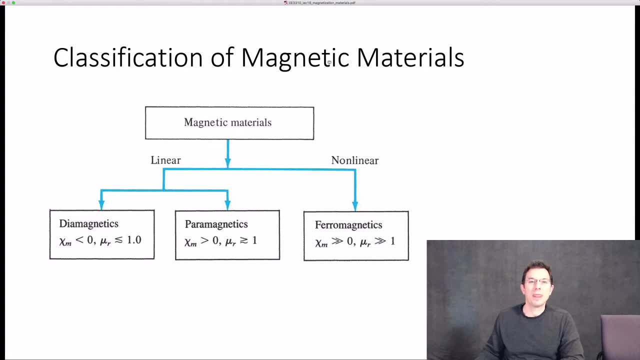 which is also equal to the permeability divided by the permeability of free space. It's just that ratio. There are several classes of magnetic flux density And this is important to understand. There are many different magnetic materials because the magnetism arises from different mechanisms. 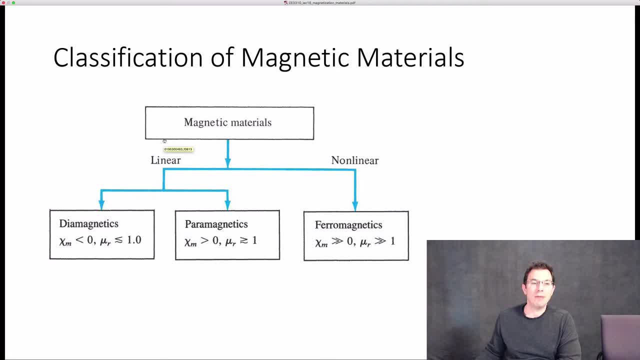 The first major division is between linear magnetic materials and nonlinear magnetic materials. Linear magnetic materials come in two kinds: One is called diamagnetic materials and the other is called paramagnetic. We'll discuss briefly the difference between those two. And then you have a class of nonlinear magnetic materials which are called ferromagnetics. 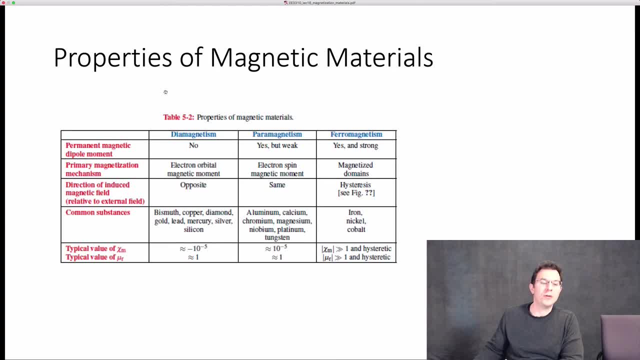 Okay. Well, what's the difference between these three different kinds of magnetic materials: diamagnetic, paramagnetic and ferromagnetic? The first major difference is the question of: does the material itself have a permanent diameter? Does it have a permanent dipole moment? 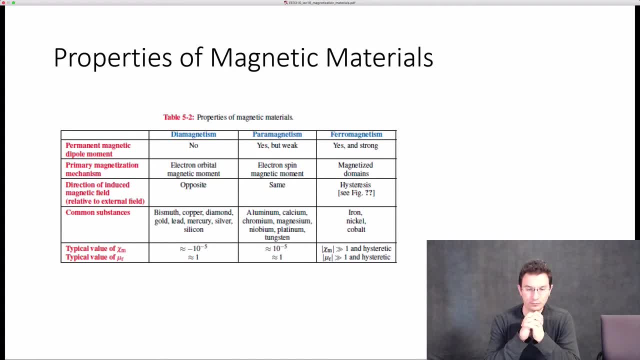 If you remember, when we talked a little bit about electrostatics, we mentioned that water molecules have a permanent electric dipole. moment, right, You've got two hydrogens attached to an oxygen. The oxygen attracts the electrons somewhat more than the hydrogen. 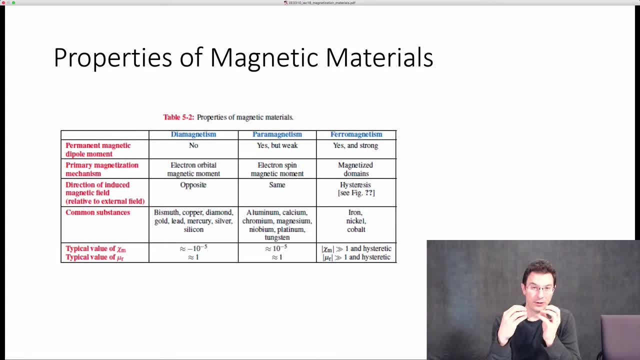 So the hydrogen side is positively charged, The oxygen side is negatively charged, And so you get a little dipole moment there that points from the hydrogens down toward the oxygen. The dual of that is a magnetic, a permanent magnetic dipole moment. 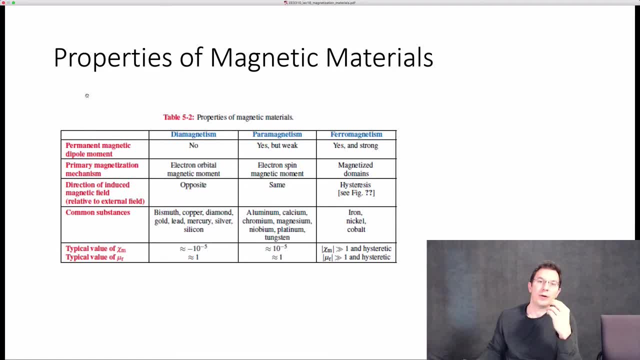 which is to say that when you don't apply a magnetic field, each of the atoms or molecules in the material still has its own little magnetic dipole moment, A permanent magnetic dipole moment. It's not induced. Diamagnetic materials do not have a permanent magnetic dipole moment. 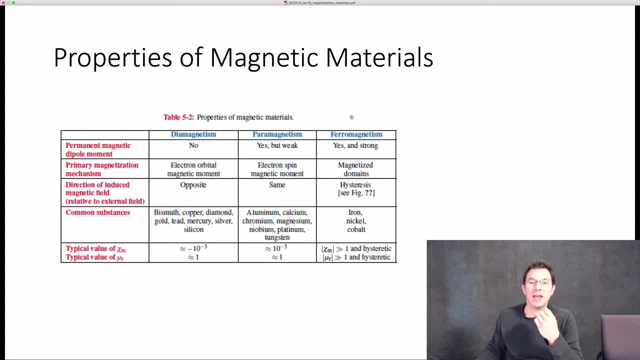 Paramagnetic materials do, but it's weak, And ferromagnetic materials have a permanent dipole moment. that's pretty strong. Diamagnetic materials get their magnetic response from the orbital, the electron, orbital magnetic momentum, In other words from the fact that 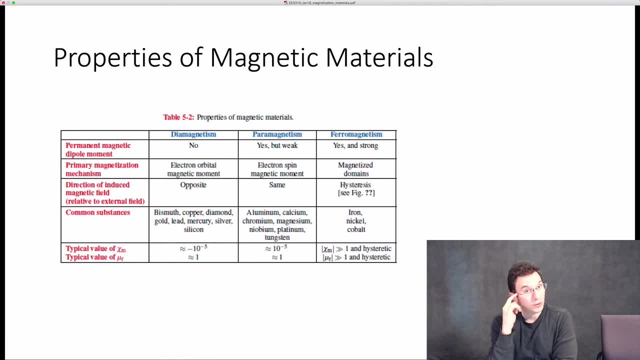 you can think about the electron orbiting the nucleus there, So that orbital angular momentum creates the magnetic response there. in a diamagnetic material, In a paramagnetic material, the magnetic response is due to the spin of the electron itself, And in a ferromagnetic material, 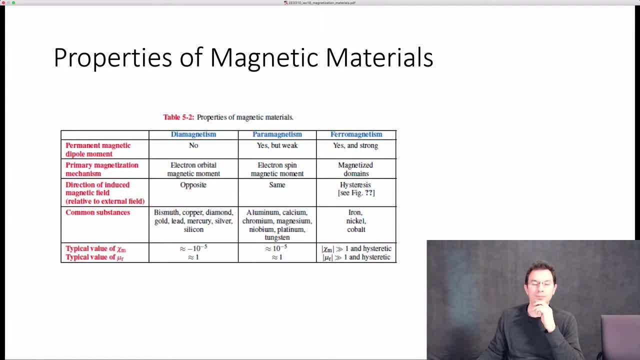 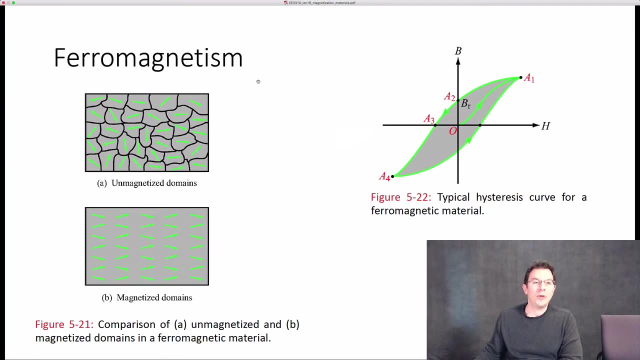 and we'll talk a little bit more about this in a moment. the origin of the magnetism is the actual magnetized domains we'll see, which are generally larger than atoms or molecules. Well, let's look a little bit here at ferromagnetism. 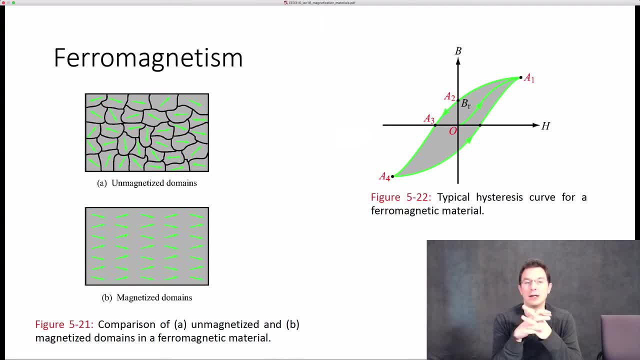 and specifically what these magnetic domains look like. Okay, It's conceptually very similar. You can see here- this is a similar picture to the one we saw earlier. You've got a whole bunch of these little magnetic dipole moments that are oriented randomly throughout the material. 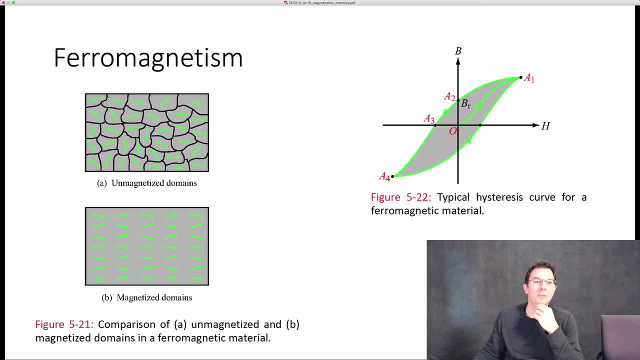 The difference is that each of these dipole moments are associated with a larger region, a larger volume. It's not just necessarily an atom or a molecule. It's many atoms or many molecules Here that each collectively have a particular dipole moment. 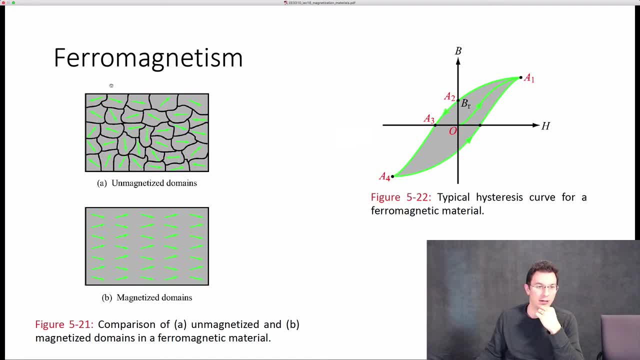 That's where ferromagnetic materials get their magnetic response. And again, if you apply an external magnetic field to this guy, the magnetic fields of all of these domains will tend to line up with the external field. That's called magnetization. Okay, 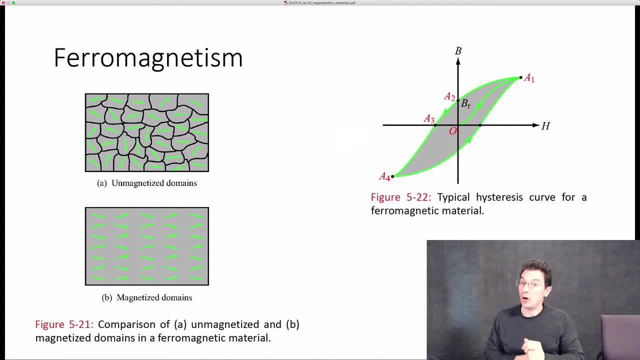 Another important property of ferromagnetic materials is that they're nonlinear, which is another way of saying there's a nonlinear relationship here between the magnetic field H and the magnetic flux density B. How does this work? Well, let's say that you've got a ferromagnetic material. 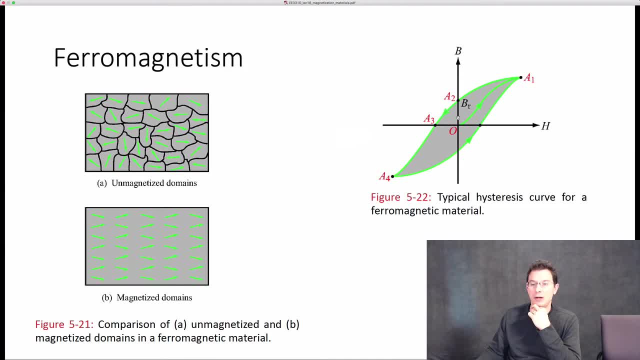 that's initially unmagnetized. So you're starting right here at the origin O. Okay, If you begin to increase the magnetic field applied to that material, the magnetic flux density will follow this path right along here up to this point A1.. 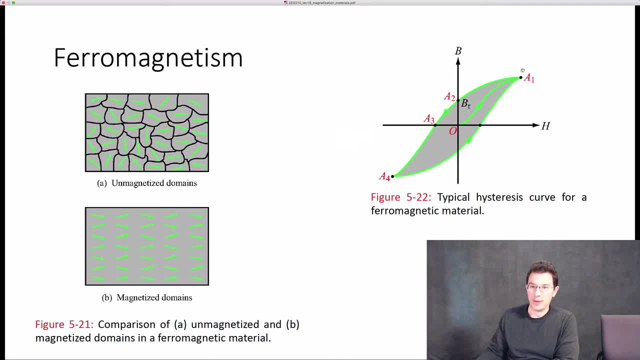 If, from there, you decrease the magnetic field, you will travel down along this path up to this point A2.. At this point A2, there's no external magnetic field anymore, And yet you still have some net magnetic flux density. That's called a magnetized state. 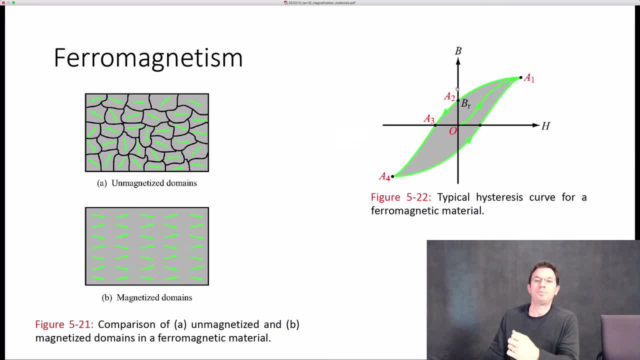 You've essentially magnetized the material at that point. If you continue to decrease the magnetic field, you get to this point A3. You're still applying a magnetic field in the opposite direction, but you're not getting any magnetic flux density. So you've essentially demagnetized the material there. 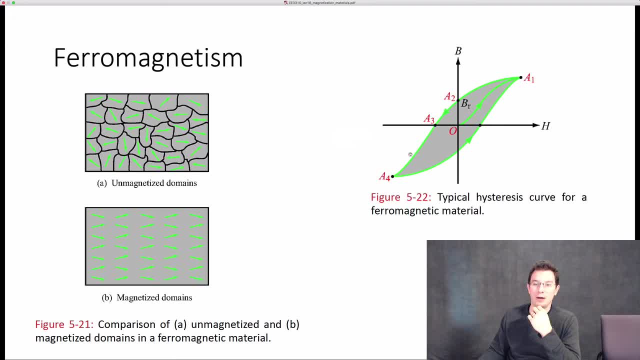 And then you're moving all the way down along this curve to A4. If you then start to increase the magnetic field again, you move up along this path back to A1 and so forth, or all the way around in a loop. This is called a hysteresis loop. 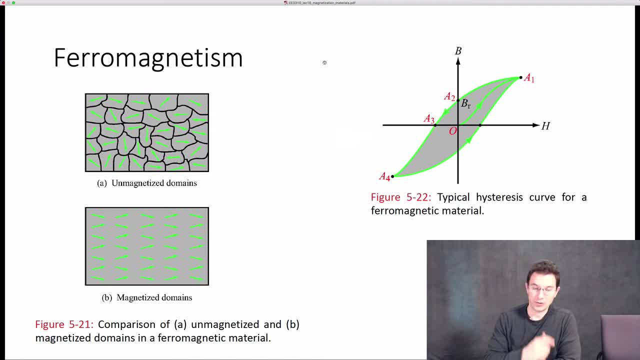 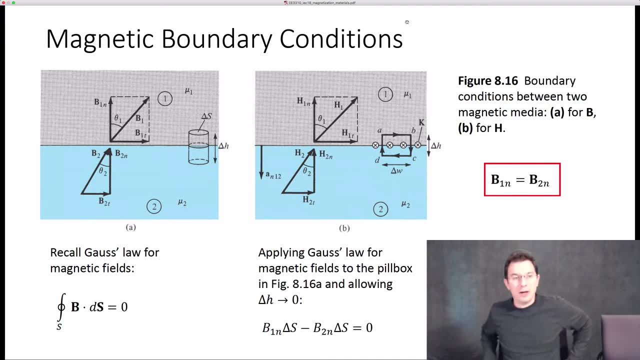 and it's characteristic of ferromagnetic materials specifically. Okay, so the second big topic we have for today is magnetic boundary conditions. We've already seen some of the electric boundary conditions and, you guessed it, they're a very similar pair of magnetic boundary conditions. 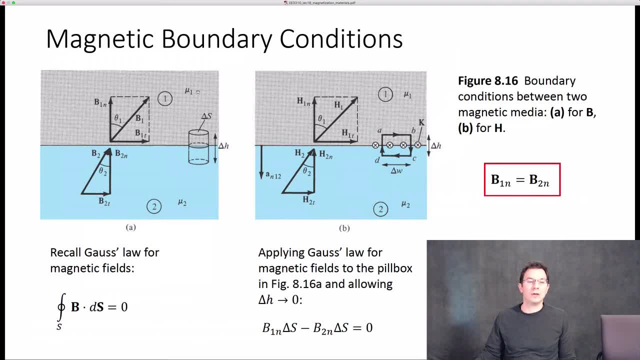 We're going to be referring to these two figures in order to derive the magnetic boundary conditions. What you're seeing here is a boundary between two different magnetic materials. This top region has a permeability mu1.. This bottom region has a permeability mu2.. 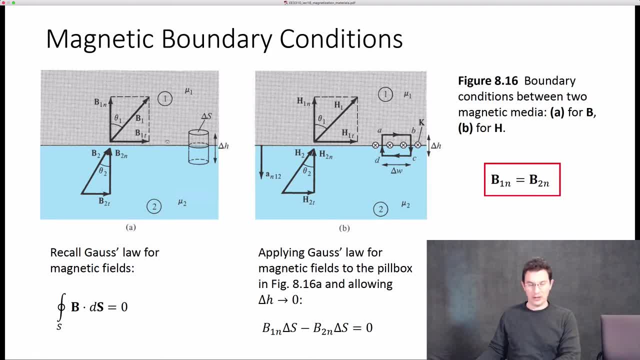 And we've got a boundary here, and so we want to know what are the equations that hold between- on the boundary, I should say, What are the relationships between the magnetic fields here on either side, evaluated at the boundary? Well, first of all, the first tool we're going to need, 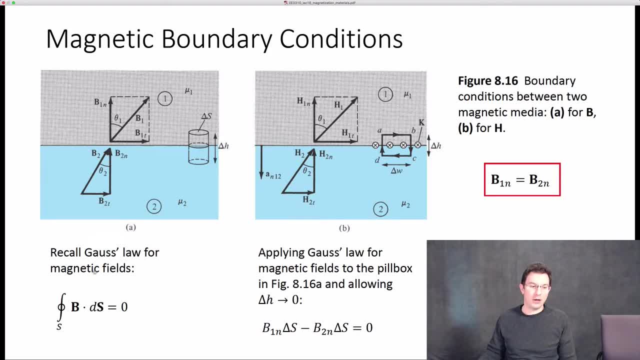 is Gauss's law for magnetic fields written in integral form here. Okay, so the surface integral of the magnetic flux, density b dotted with ds, is equal to zero. That's where we're going to start And we're going to apply Gauss's law for magnetic fields. 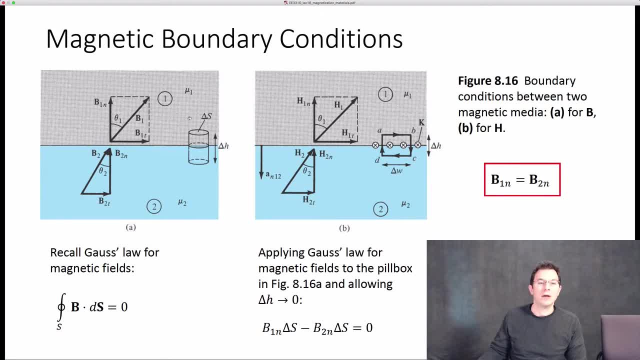 to this little pillbox right here, this little cylinder. So we're going to say that, okay, the total integration over this entire surface is equal to the integration over the surface, over the top, an integration over the sides of the pillbox. 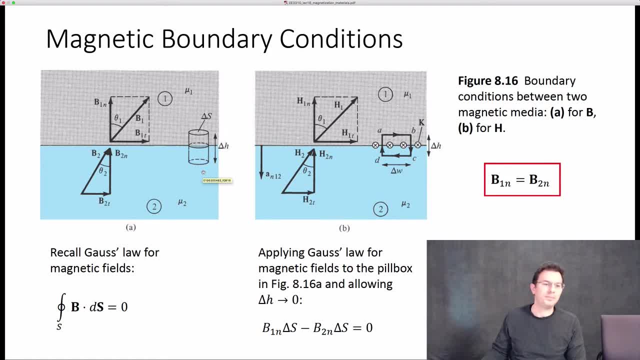 and an integration over the bottom of the pillbox. Okay, What we're going to do then? that's going to be our first move and then, after we set up the integral over the top, bottom and sides, we're going to play the game. 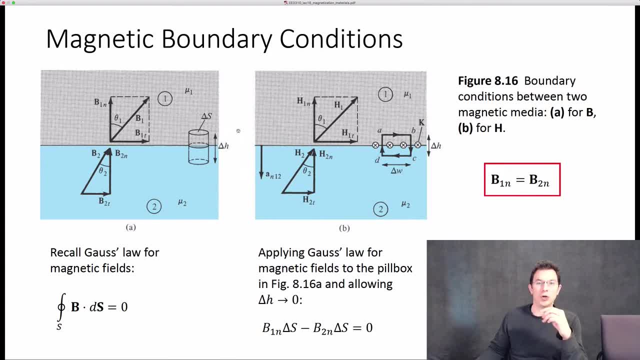 We're going to say: now let the height of this pillbox delta h go to zero. Now we're going to collapse it down until it's on the surface. That's how we're going to get. the boundary conditions was when the height of that pillbox gets to zero. 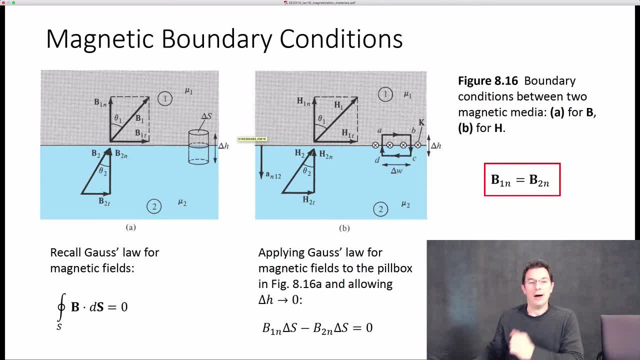 then you're on the surface, The integral. if you make this surface small enough, we can consider the magnetic field to be constant across that surface here, magnetic flux density to be constant. So what you get? the contribution from this integration due to the top surface here. 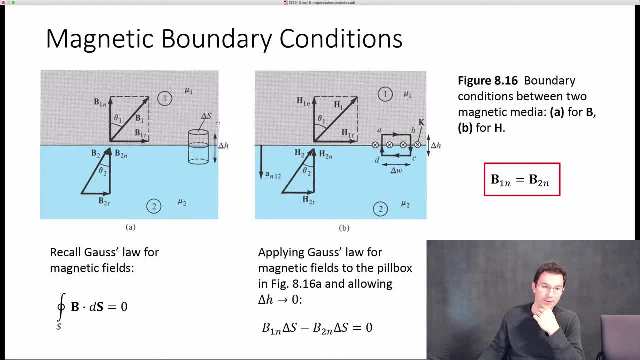 is the normal complex, the normal component of the magnetic flux density in region one that's b1n here, the normal component. right, You've got a dot product between a normal vector to that surface with the magnetic field, with the magnetic flux density. 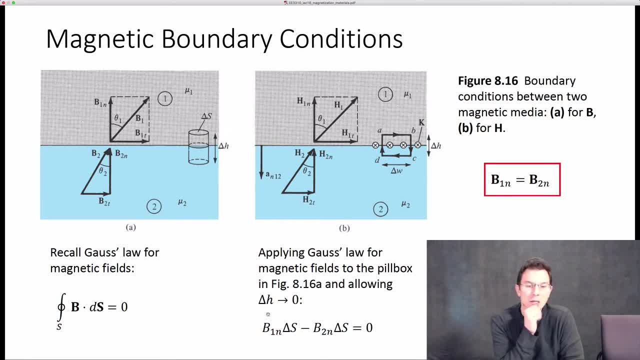 that picks out just the normal component, b1n times the area delta n, that's on the top, minus due to the downward pointing surface normal there, because all the surface normals point out of the volumes minus the normal component of the magnetic flux density. 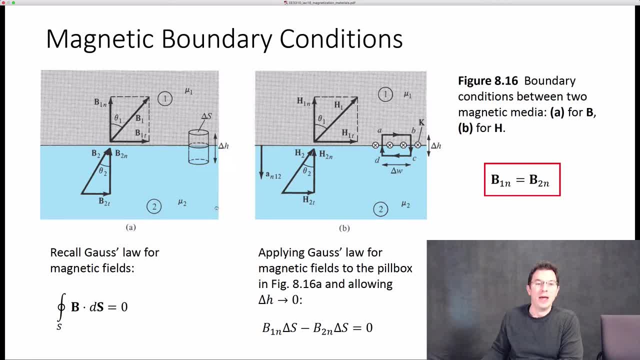 in region two times that area and the integrals over the sides have gone to zero, because you get the normal component of the magnetic flux: density here times the surface area of that surface, the outer surface, which is related to the height, delta h. 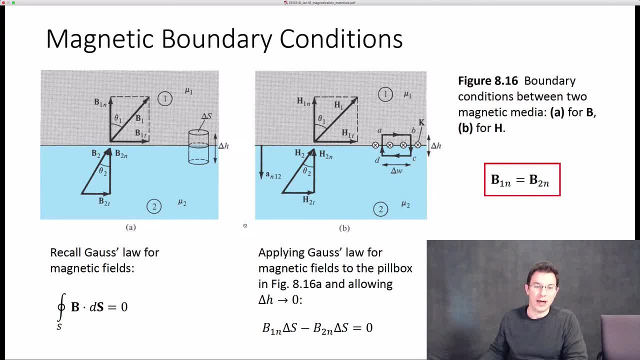 As delta h goes to zero, that term falls out and the only thing that remains is this equation right here, which comes from Gauss's law for magnetic fields: Solve both sides, for I should say: add b2n, delta s to both sides. 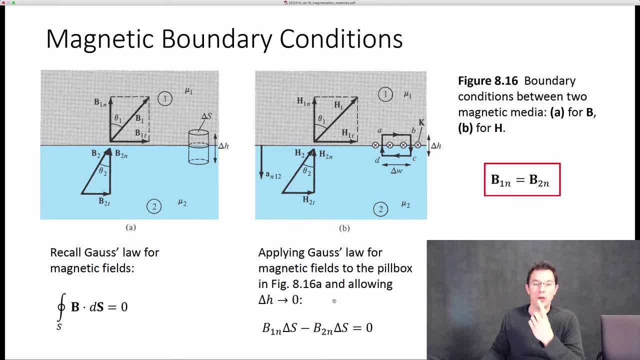 cancel out the delta s's and it turns out that the normal component of the magnetic flux density is continuous across the surface. In other words, it is equal. they are equal at the surface. the normal component of the magnetic flux density must be the same. 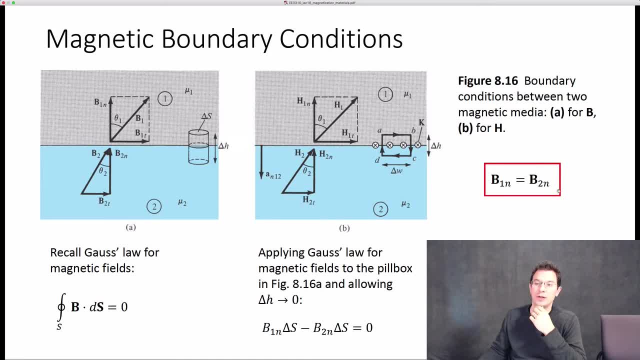 And that is written, that's expressed here by this equation: The normal component of the magnetic flux, density, is equal on the surface of the, on the interface, on the surface there. That's one of our two boundary conditions. We've got one of two done. 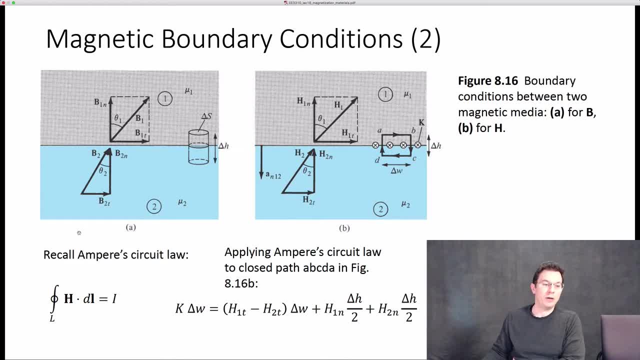 The next boundary condition. we need a different starting place for that, and the starting place for that one is Ampere's circuit law or Ampere's law in integral form right here, Integral around any closed loop. L of h dot dl is equal to the current enclosed by that loop. 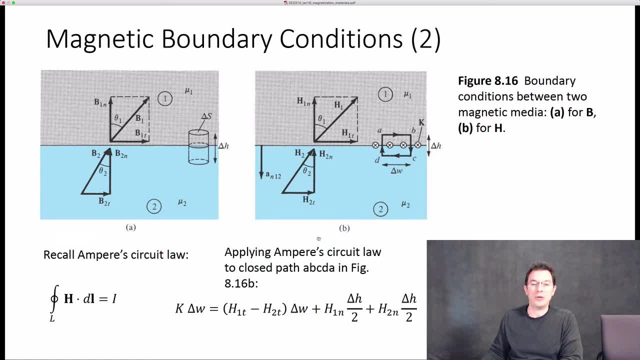 Okay, what we're going to do next is we're going to apply Ampere's circuit law to a closed path a, b, c, d, a in figure 816b right here. So here's the path that we're going to. 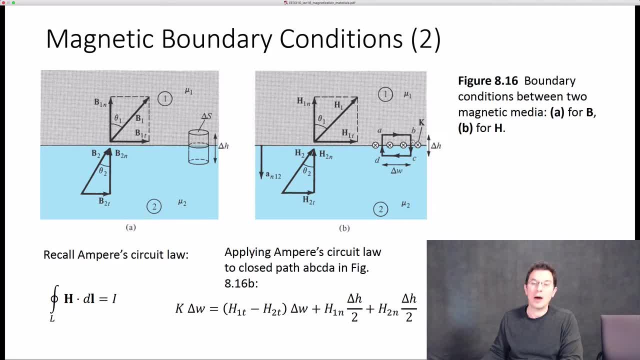 this is going to be our L, our capital L, right here. This is the path around which we are going to apply Ampere's circuit law. Okay, by similar arguments, I'm going to say: if the path gets short enough, I can approximate the tangential component here. 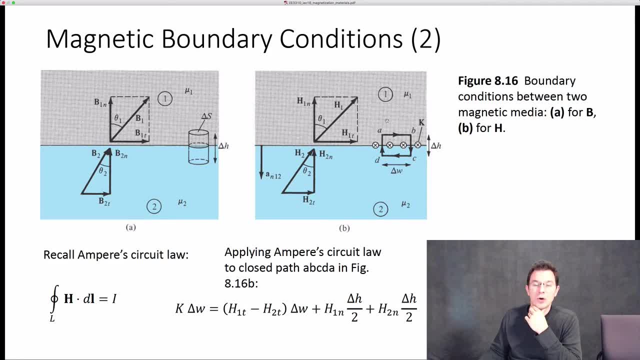 of each vector as constant. So when I take a dot product with dl along this path, I take a dot product between dl along that path and h. I'm going to get the tangential component of h here in region 1, because we're in region 1.. 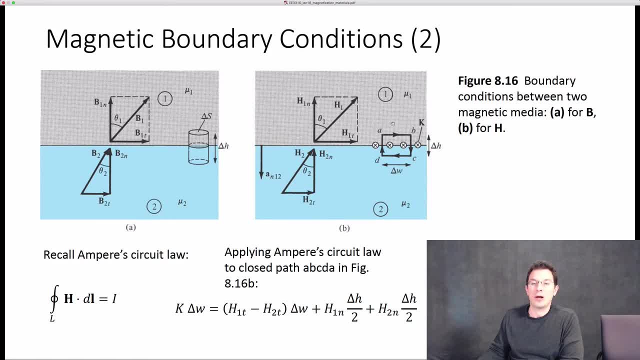 So we've got h1t, the tangential component of h in region, 1, times this distance. that's delta w that comes from this line integral. So that's this term: h1t times delta w. That comes from that first dot product in integration. 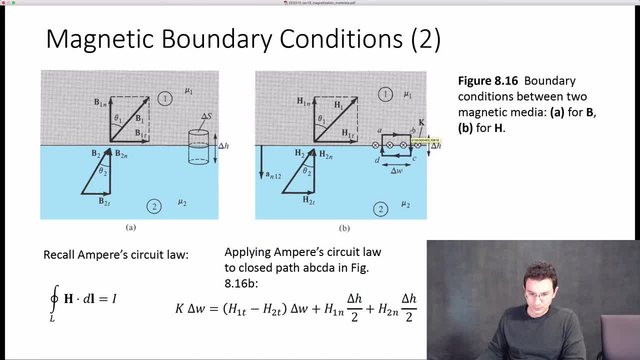 And then I've also got a couple of other pieces here. If this distance is delta h, I'm also going to be picking out the normal component in region 1 from here and here- Okay, right, there and there, And I'm going to get the normal component. 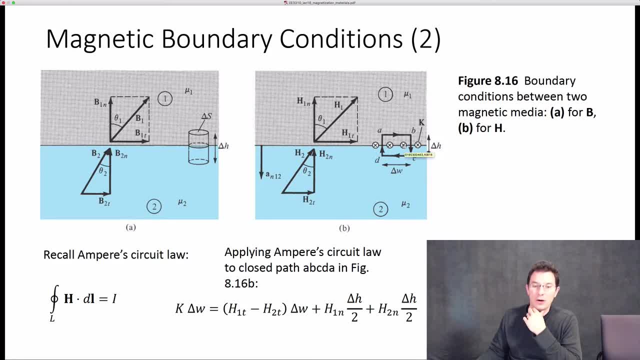 in region 2 from here and here. Okay, that's where these two, these two terms come from. Again, you get the normal component, because this line segment is normal at 90 degrees to the interface. And then, how much? how much current am I enclosing here? 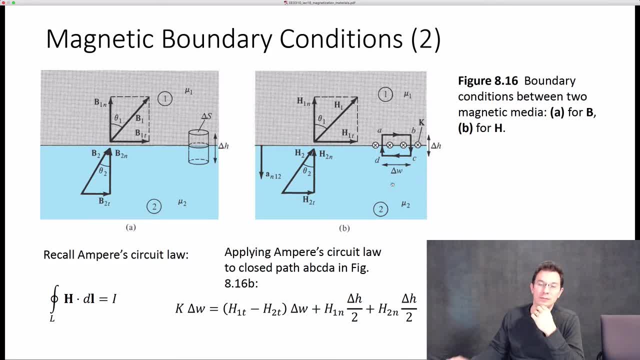 Well, again, if delta h is small enough, the only current that can exist is right there on the surface. So we have a surface current density k times the length of the surface enclosed by this thing. that's delta w right here. 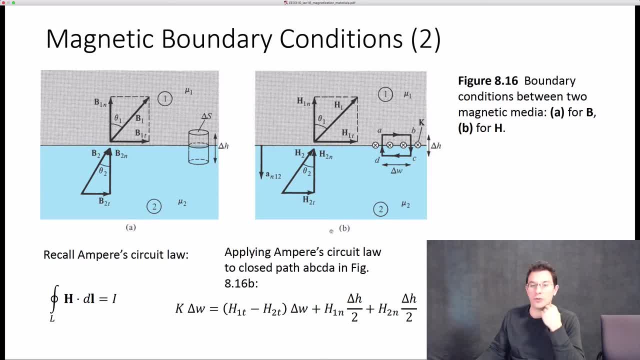 And this actually is I. This is the amount of current that's enclosed by this path. I'm going to play the same game. I'm going to allow this delta h distance to go to 0.. If I do that, clearly these two terms fall out.